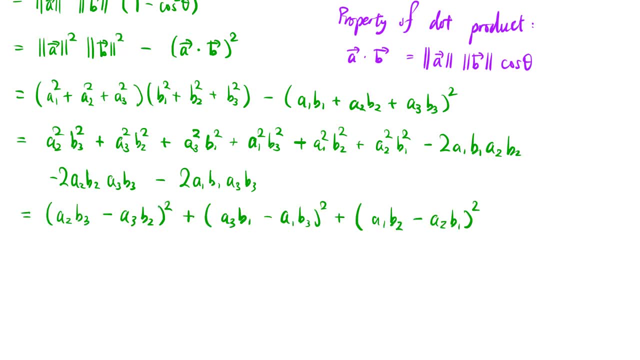 the square of A2- B3 minus A3 B3.. The square of A2- B2 plus the square of A3 B1 minus A1 B3, plus the square of A1 B2 minus A2 B1.. And this is equal to the square of length of A cross B. 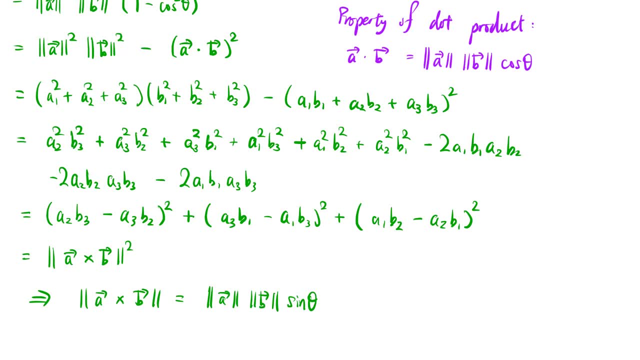 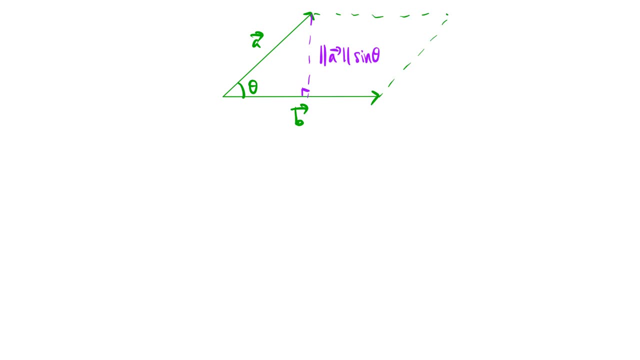 Hence the length of A cross B equals the length of A times the length of B times sin theta. Now we consider the parallelogram formed by A and B. By taking the length of B as the base, we know that the height is equal to the length of A. 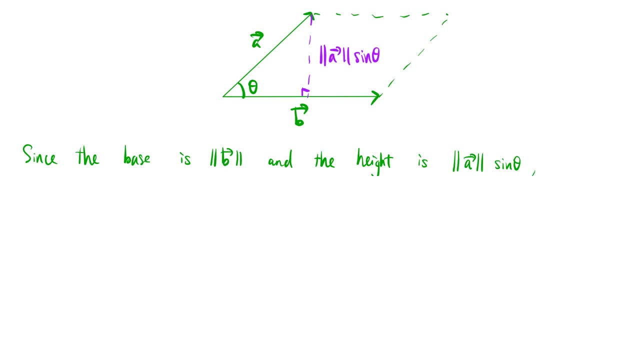 times sin theta, using simple trigonometry. Hence, the area of the parallelogram equals the length of B times the length of A times sin theta, which equals the length of A times the length of B times sin theta, And this completes the proof. 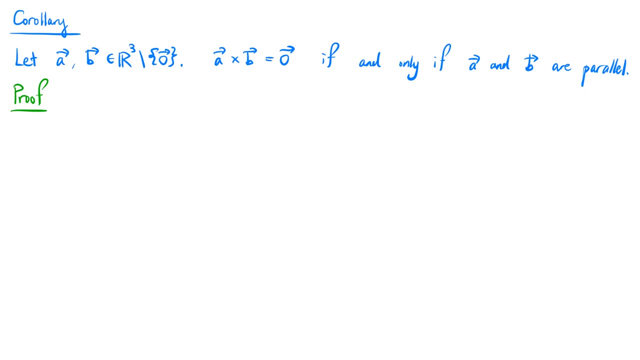 Let's look at a corollary of this result. Let A and B be non-zero vectors in R3.. Then A cross B equals the zero vector. if, and only if, A and B are non-zero vectors, Then A cross B equals the zero vector if, and only if, A and B are non-zero vectors. 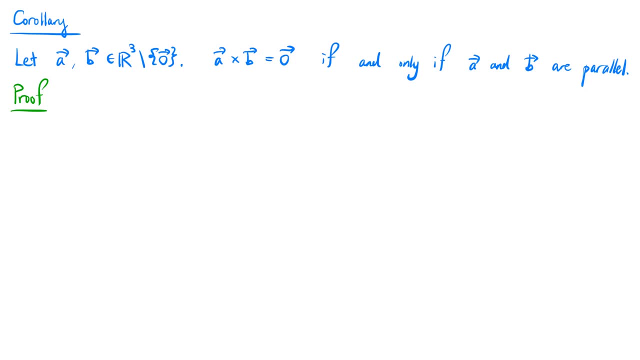 if a and b are parallel. For the proof, a cross b equals the zero vector. if, and only if, the length of a cross b equals zero. From the previous result, this happens if, and only if, the length of a times the length of b, times sine theta, equals zero, Since the length of a and the length of b are non-zero. 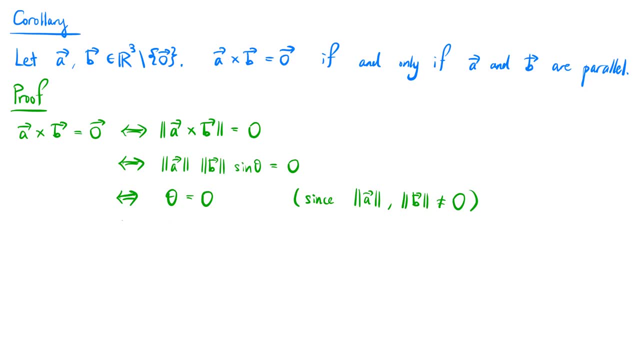 this happens if, and only if, theta equals zero, In other words, a and b are parallel. Let's look at an example. Suppose we want to find the area of the triangle in R3 with vertices and let a be the vector 1, 1 0 minus 1 0. 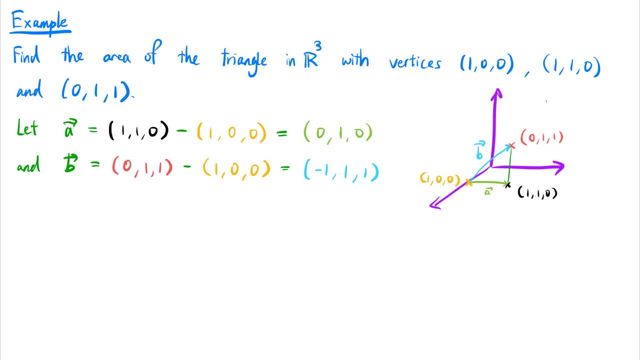 0, which equals 0 1 0.. Let b be the vector 0 1 1 minus 1 0 0, which equals negative 1 1 1.. Note that all of the vectors which correspond to thesevector are nearly equal to the range of interaction or olmazings. but the distance between players and attack the string is 2000 degrees depending on the area. Now recognise a vector 0. this was dc. there are 5 elements here. Notice that a, минe and b are parallel. there are no significant differences between the middle and the other. all of the verticals. 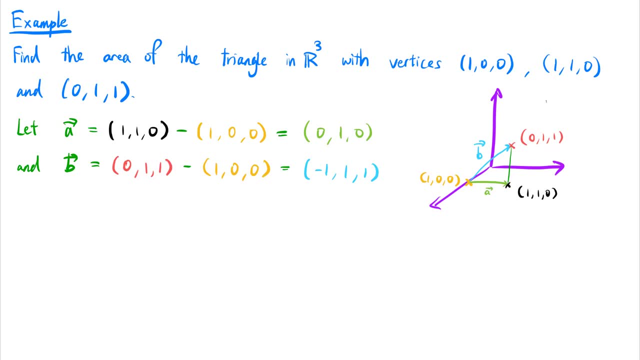 Notice that the meter width is 2 by i M1, V1, 3 p 봉 and i M2?. In addition, these are all the same that the lengths of these two vectors are equal to the lengths of two sides of the triangle. 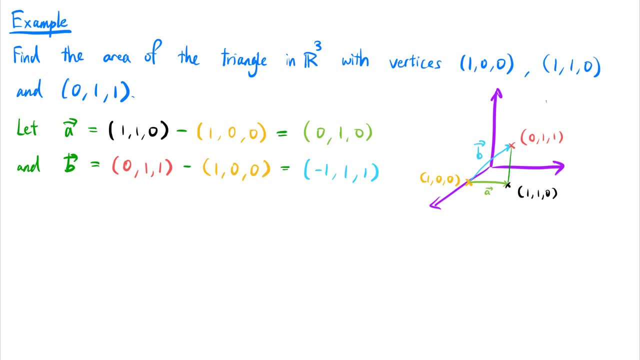 To find the area of the triangle, it suffices to find the area of the parallelogram formed by a and b and divide by 2, which in turn can be found by computing the cross product of a and b. So we compute a cross b equals the determinant of e1, e2, e3, 0, 1, 0, negative 1, 1, 1.. 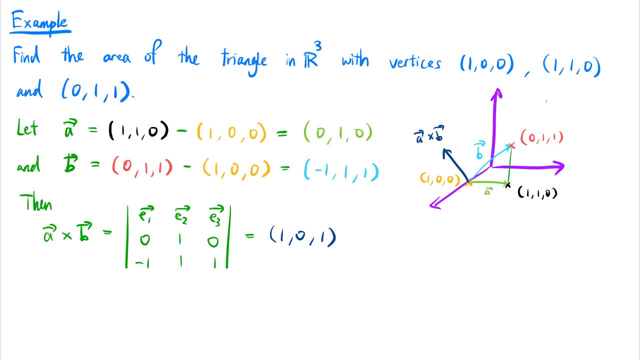 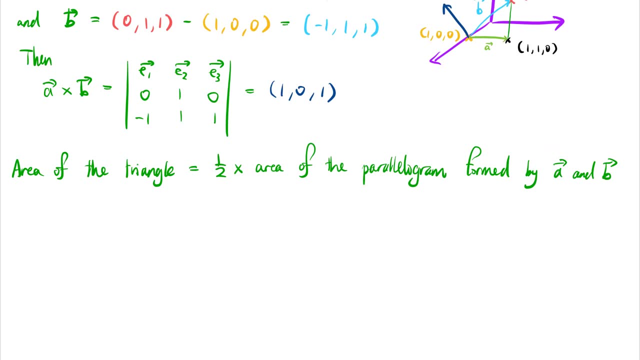 This equals the vector 1, 0, 1.. Hence, the area of the triangle is equal to one-half times the area of the parallelogram formed by a and b, which equals one-half times the length of a cross b. This equals to one-half times the square root of 1 squared plus 0 squared. 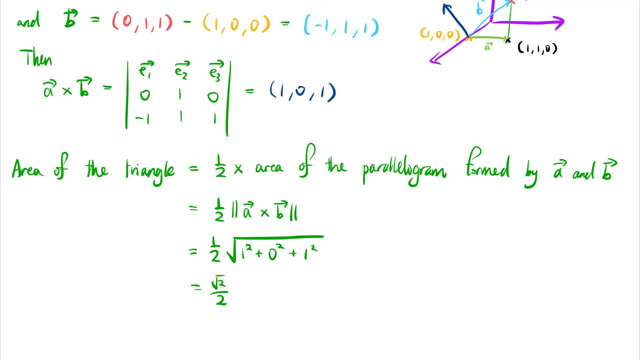 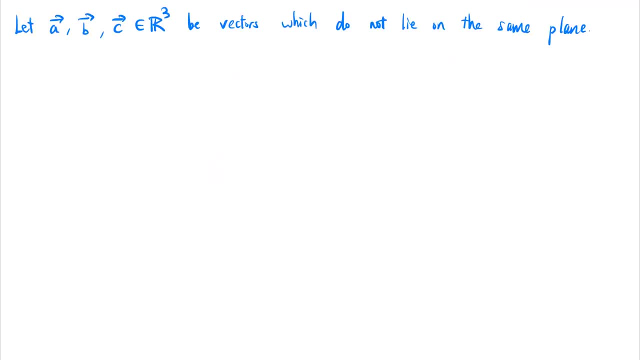 plus 1 squared and we get the answer square root of 2 over 2.. Now let's consider vectors a, b, c in R3, which do not lie on the same plane. They determine a solid called a parallelepiped. 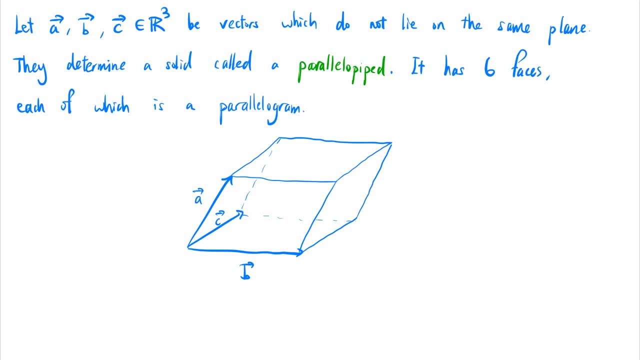 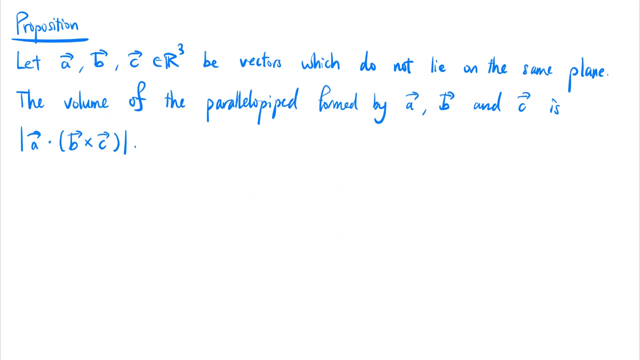 It has six faces, each of which is a parallelogram. This is a generalization of the fact that two vectors form a parallelogram. Let's look at a proposition. Let a, b, c be vectors in R3 which do not lie on the same plane. 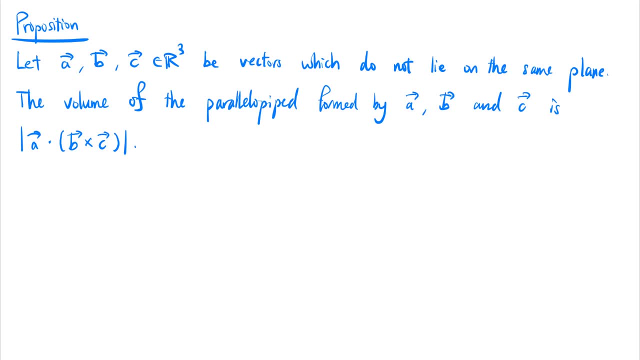 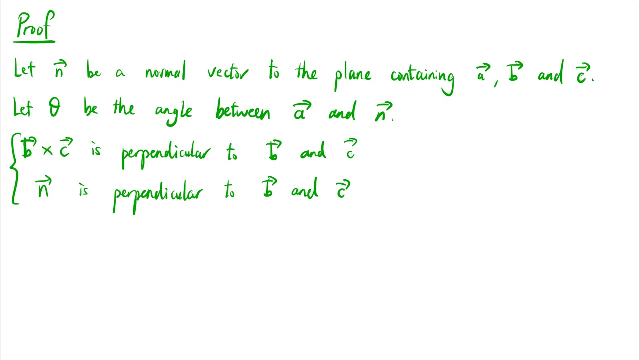 The volume of the parallelepiped form b- c is equal to the absolute value of a dot-bracket b cross c. For the proof, let n be a normal vector to the plane containing a, b and c. Let theta be the angle between a and n. We know that b cross c is perpendicular to b and c. 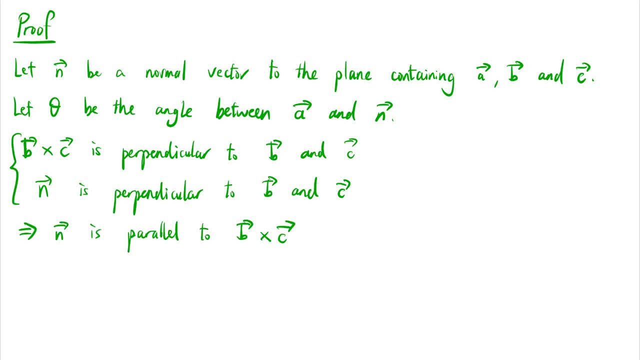 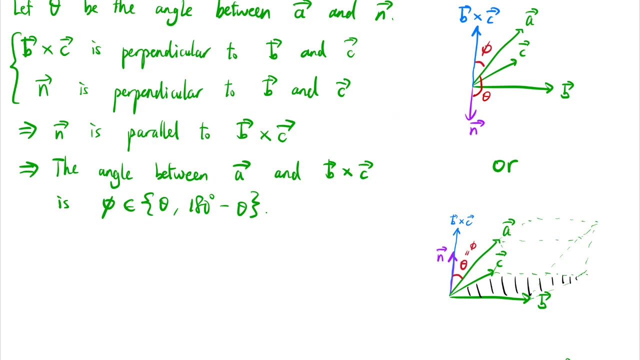 and also n is perpendicular to b and c. So n is parallel to b cross c. between A and B cross C is phi, which is either theta or 180 degrees minus theta. Now the volume of the parallelepiped is equal to the base area times the height where the 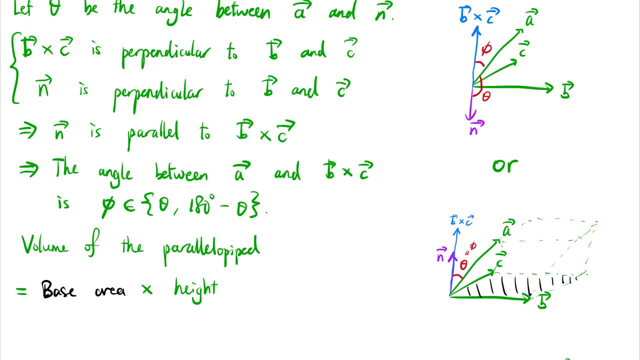 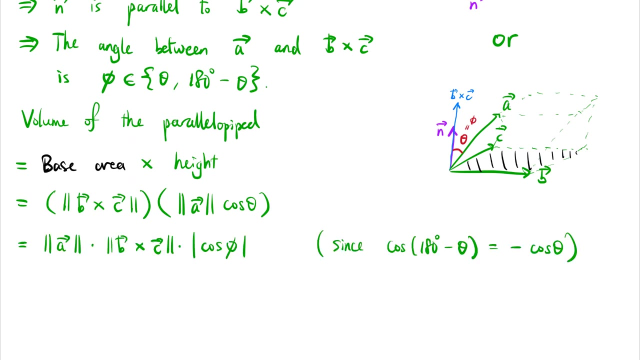 base area is the area of the parallelogram formed by B and C, which is the length of B cross C and the height is equal to the length of A times cos theta. Since cos of 180 degrees minus theta equals negative cos theta, we can rewrite cos theta: 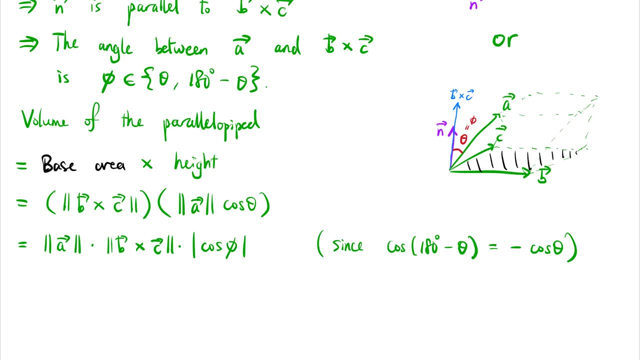 as the absolute value of cos phi, because cos phi is equal to cos theta or negative cos theta. so the expression becomes the length of A times the length of B cross C times the absolute value of cos phi. This is exactly equal to the absolute value of A dot bracket B cross C. 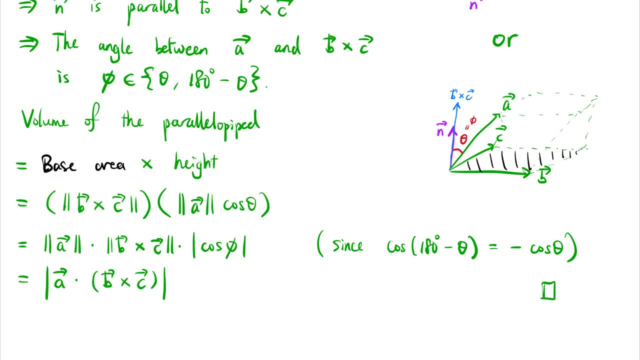 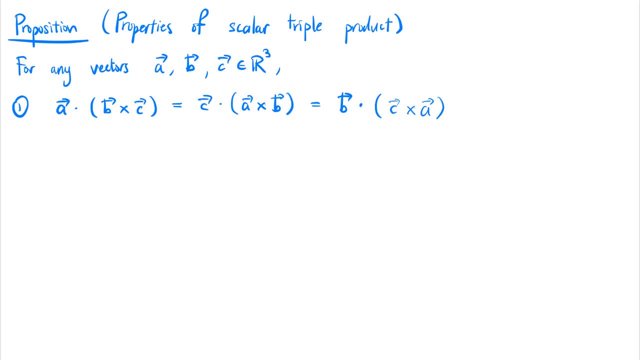 And this completes the proof. Now let's talk about some properties of the scalar triple product. For any vectors A, B and C in R3,: A dot B cross C equals C. dot A cross B equals B. dot C cross A. 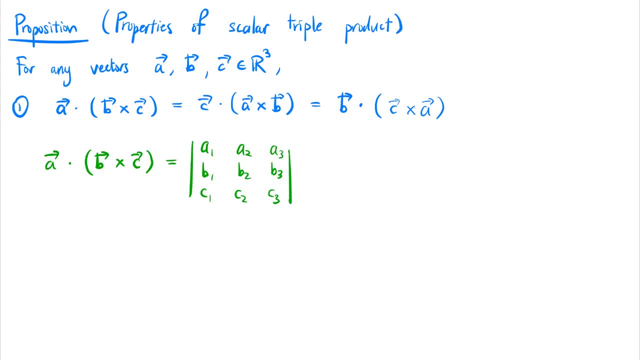 We write: A dot, B cross. C equals the determinant of A1, A2,, A3,, B1, B2, B3,, C1,, C2, C3.. We swap the second and the third rows to give the negative of the determinant A1, A2, A3,. 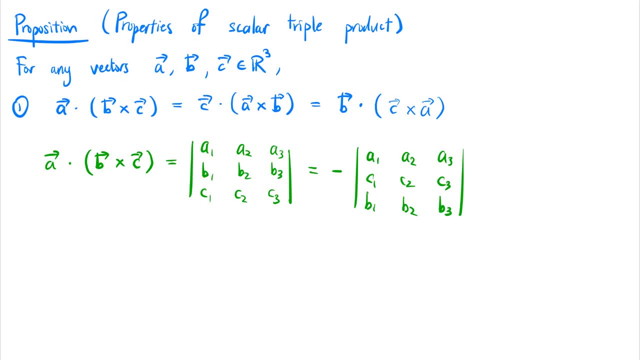 C1, C2, C3,, B1, B2, B3.. Now we swap the first and the second rows to give the determinant of C1, C2, C3,, A1,, A2,, A3,, B1,, B2, B3, which is equal to C, dot A cross B. 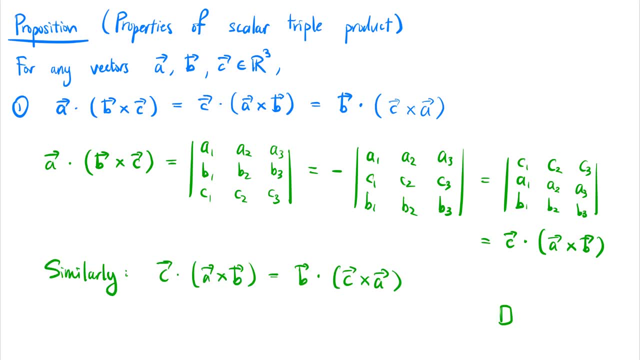 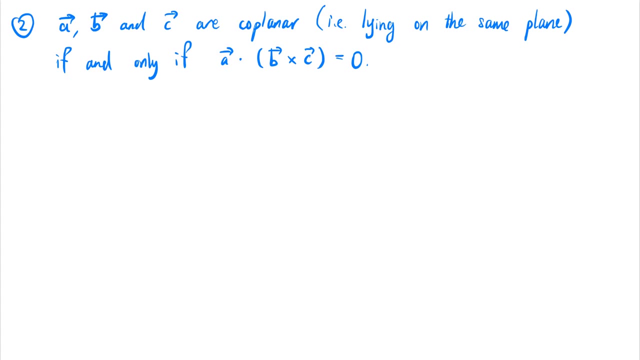 Similarly, by swapping two rows of the determinant twice, we have C dot A cross B equals C dot A cross B. The second property, A, B and C are coplanar, in other words lying on the same plane. if 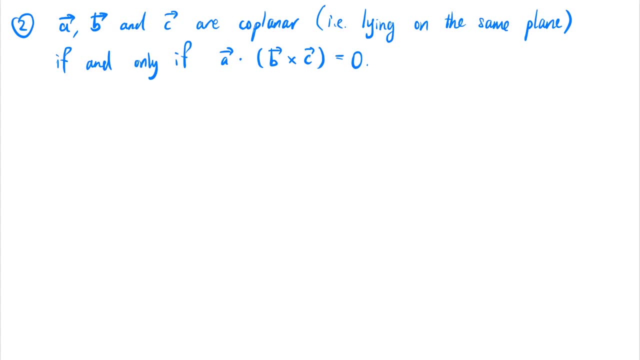 and only if, A dot B cross C equals 0.. Indeed, A, B and C are coplanar if, and only if, the volume of the parallelepiped formed by A, B and C is 0.. Using the previous result, this happens if, and only if, A dot B cross C equals 0. 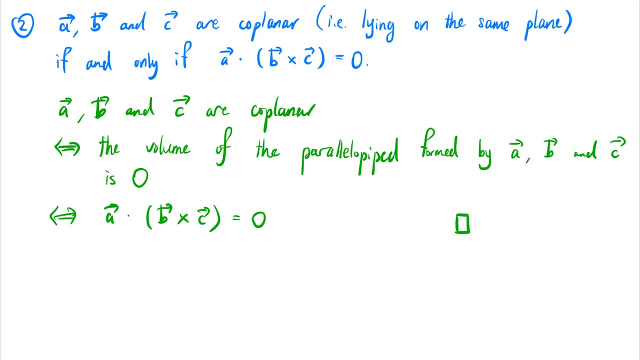 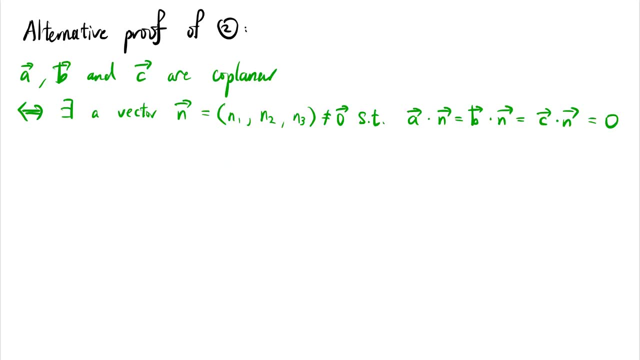 Alternatively, we can prove the second property as follows: A, B and C are coplanar if, and only if, there exists a vector n in the form n1, n2, n3, which is non-zero, such that A dot n equals B, dot n equals C dot n equals 0.. 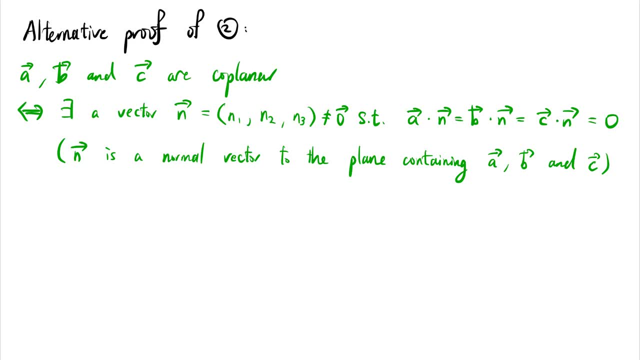 Here n is a normal vector to the plane containing A, B and C. This happens if, and only if, A dot B cross, C equals 0. Similarly, if the homogeneous system A1, A2,, A3,, B1, B2,, B3,, C1,, C2, C3 times n1,, n2, n3. 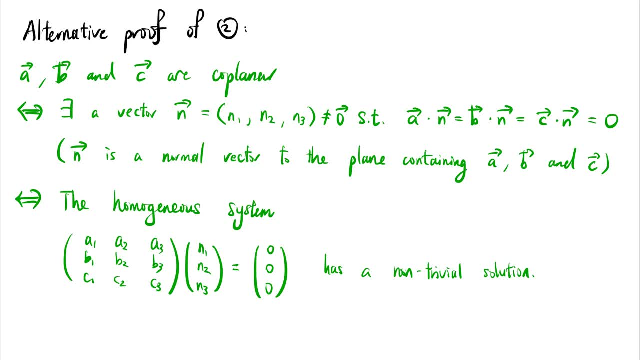 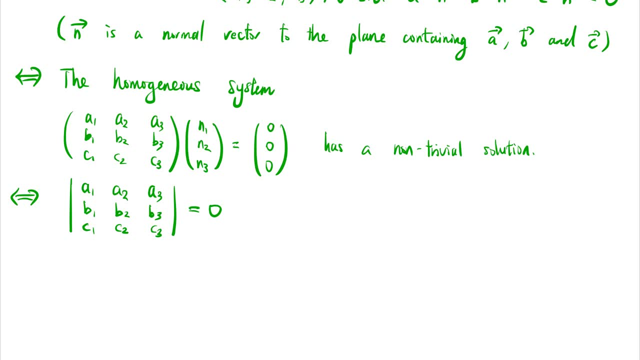 equals the zero vector has a non-trivial solution. This happens if, and only if, the determinant of the coefficient matrix A1, A2,, A3,, B1,, B2,, B3,, C1,, C2,, C3 is 0, which in turn happens if, and only if, A dot B cross C equals 0.. 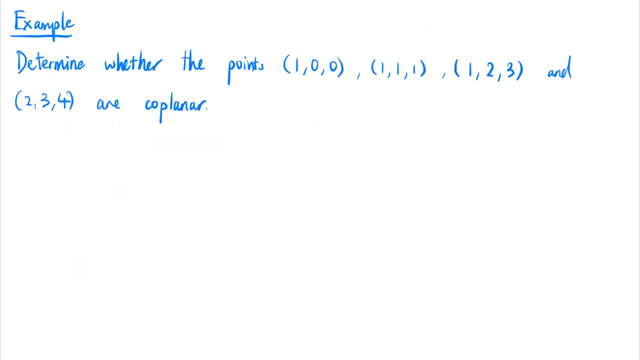 Let's look at an example. Suppose we want to determine whether the points 1, 0, 0, 1, 1, 1, 1, 2, 3, and 2, 3, 4 are coplanar. 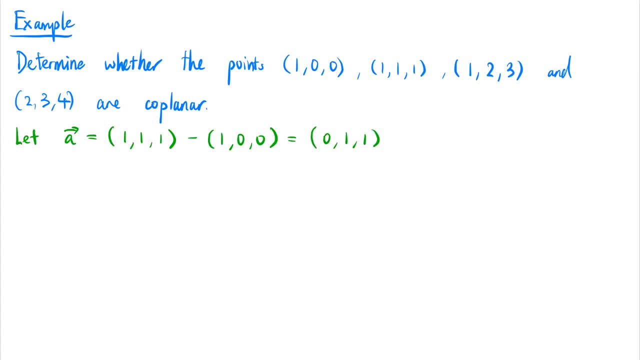 Let: A equals 1, 1, 1 minus 1, 0, 0,, which equals 0, 1, 1.. B equals 1, 2, 3 minus 1, 0, 0,, which equals 0, 2, 3.. 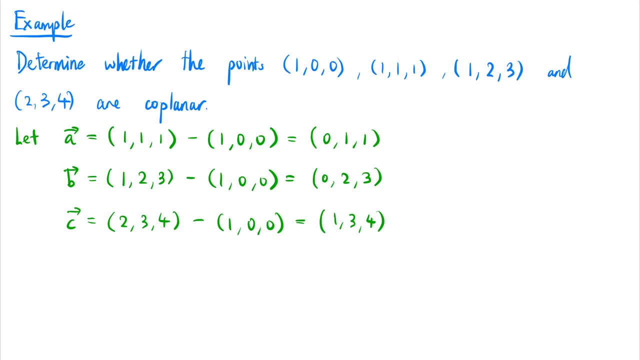 C equals 2, 3, 4 minus 1, 0, 0 equals 1, 3, 4.. These three vectors originating from the same point form a parallelepiped, and its volume tells us whether the four points are coplanar. 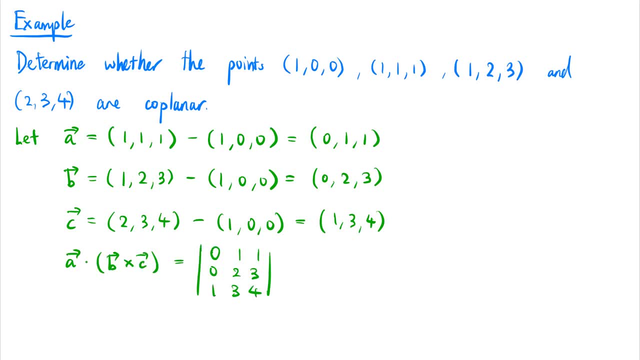 So we compute A, dot B, cross C, which equals the determinant of 0, 1, 1, 0, 2, 3, 1, 3, 4.. Expanding along the first column, we get 1 times the determinant 1, 1,, 2, 3.. 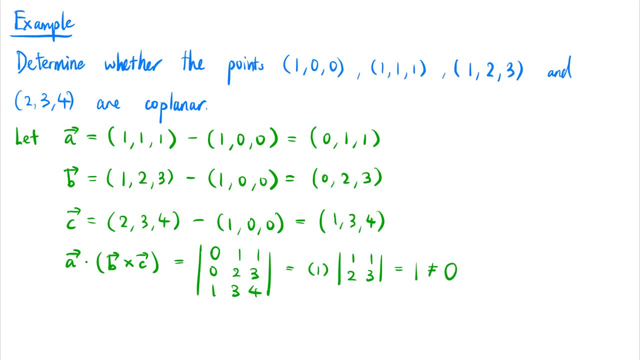 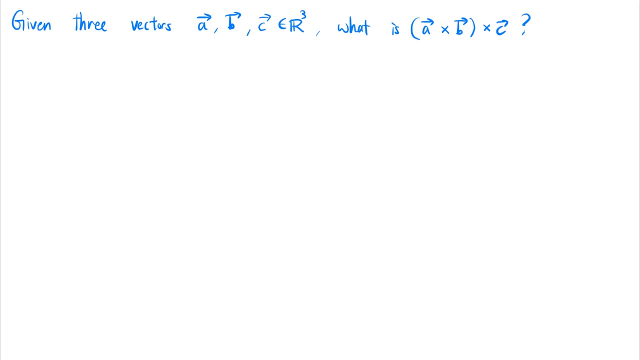 This equals 1, which is non-zero. So the volume of the parallelepiped formed by A, B and C is non-zero, which means that the four points are not coplanar. Given three vectors- A, B and C- in R3, what is bracket? A cross B, cross C. 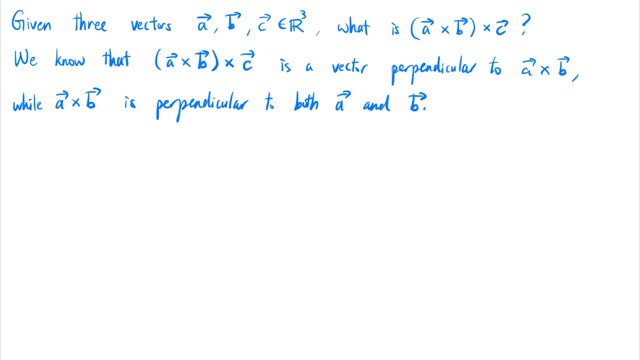 We know that bracket A cross B cross C is a vector perpendicular to A cross B, while A cross B is perpendicular to both A and B. Hence, bracket A cross B, cross C is parallel to the plane containing A and B. In other words, bracket A cross B, cross C lies on a plane containing A and B. 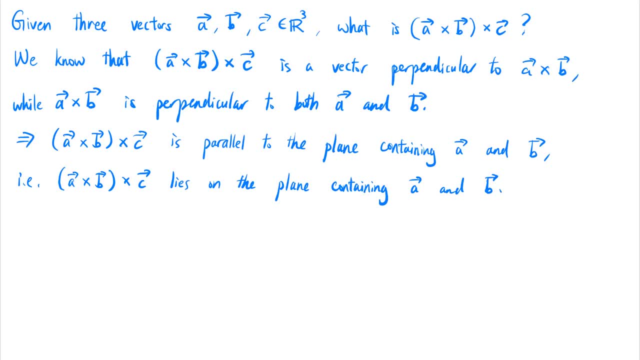 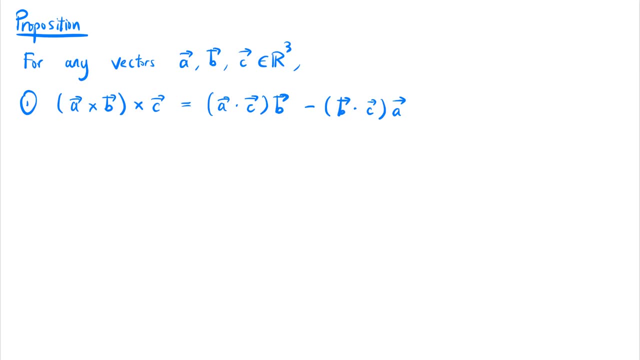 The following proposition gives the exact expression of this vector For any vectors A, B and C in R3, bracket A cross B cross C equals bracket A dot C times B, minus bracket B dot C times A. We let A equals A1.. 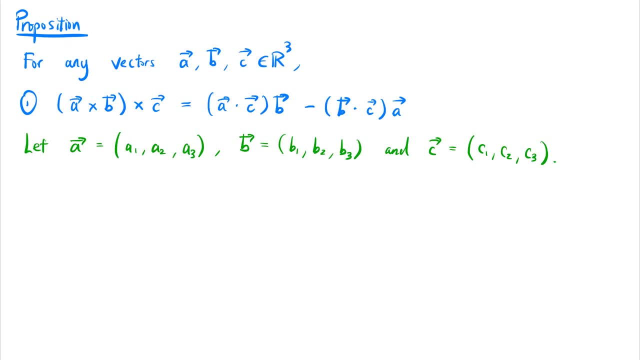 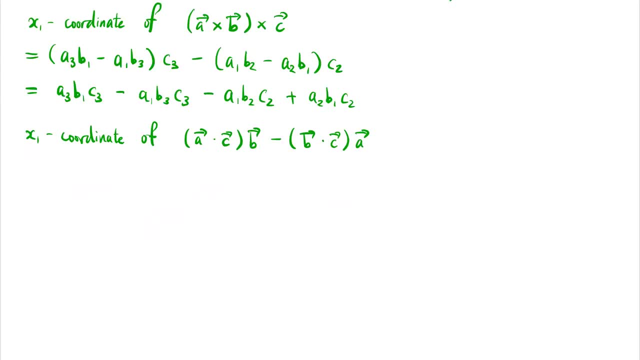 c2.. On the other hand, the x1 coordinate of bracket a- dot c times b minus bracket b dot c times a, equals bracket a1, c1 plus a2, c2 plus a3, c3 times b1 minus bracket b1, c1 plus b2, c2. 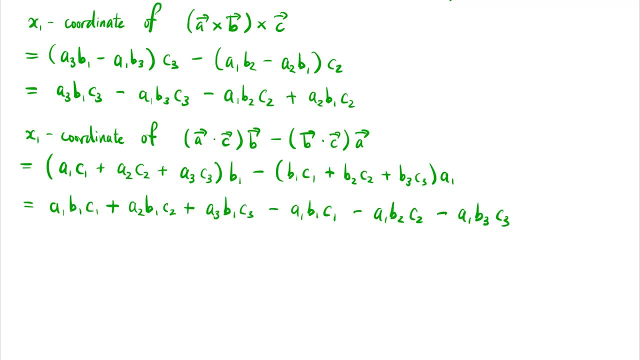 plus b3 c3 times a1.. This equals a1 b1- c1 plus a2 b1 c2 plus a3 b1- c3 minus a1 b1 c1 minus a1 b2 c2 minus a1 b3- c3.. This equals a3 b1- c3. 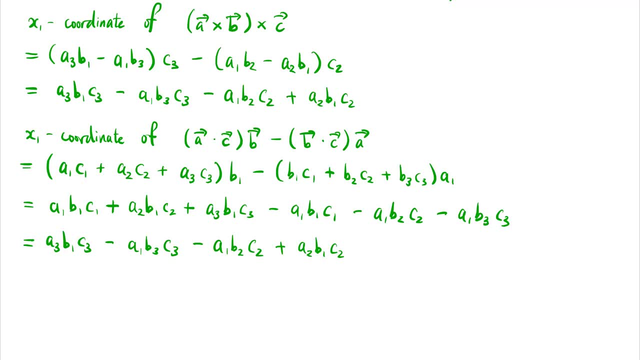 minus a1- b3, c3,. minus a1- b2, c2,. plus a2- b1, c2,. so the two expressions are equal. Similarly, the expressions for the x2 coordinates and x3 coordinates are equal, so the two vectors are equal. 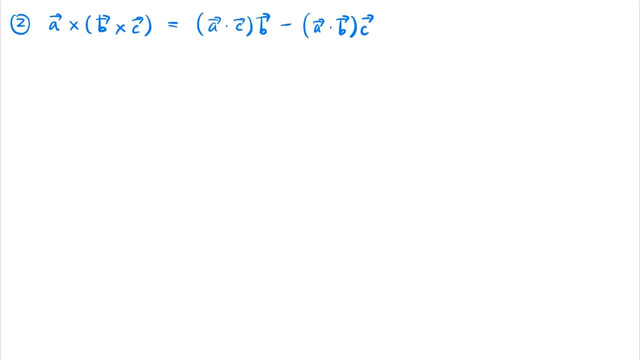 Secondly, a cross bracket b cross c equals bracket a dot c times b, minus bracket a dot b times c. We can make use of the first point and the properties of the factor product to prove this result more quickly. a cross bracket b cross c equals the negative of the vector. bracket b cross c cross a.